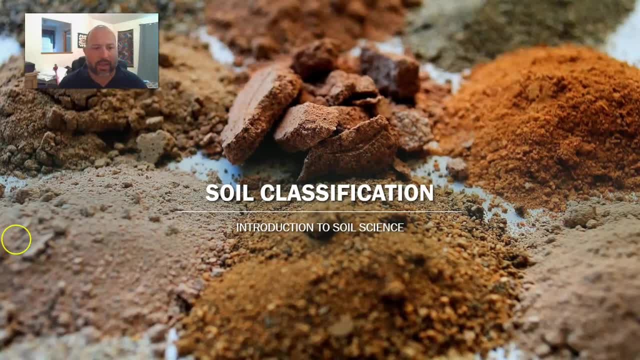 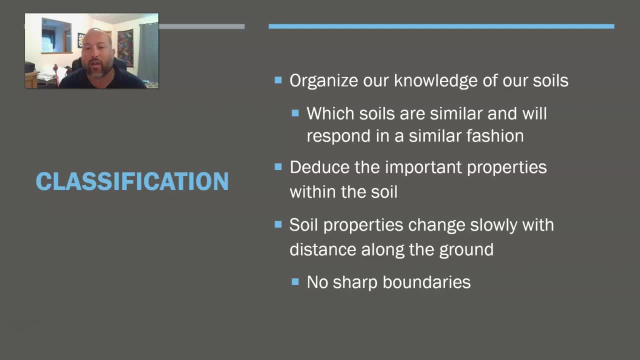 Hello everybody. so let's talk about some soil classification. So with the idea of classification, really we want to organize our knowledge of soils, So just trying to put soils together that are similar, similar in look, similar in properties and are going to respond to the type of management that we do in similar fashion. 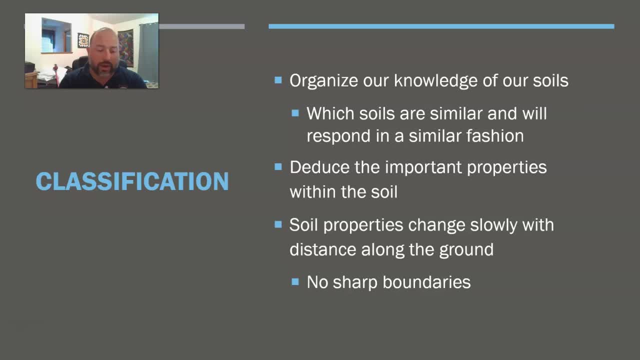 We also want to be able to figure out what's important about the soil, or what's important within the soil, or what are the important properties within the soil. Why group these together? So what about these soils? should make them a group, And the easiest way to think about that is: what are the properties within the soil that make them the same? 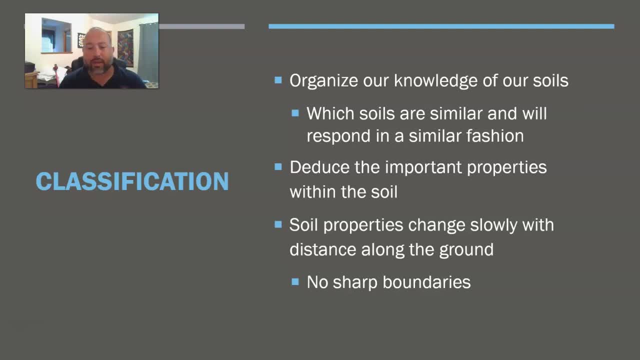 The hard part about that is soil properties change slowly with distance along the ground, So sometimes it's obvious that they're the same. Sometimes it's not very obvious. There's no sharp boundaries and there's no real big cutoff point. So we've got to kind of just figure it out and we've got to come up with a classification system that works for us. 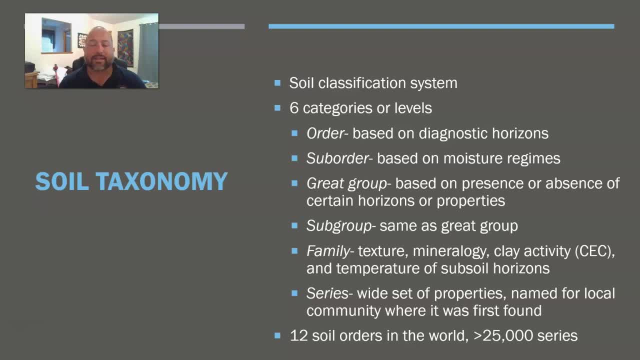 And so the one that we've come up with is soil taxonomy. It's got six categories or level, with our highest level being order and our lowest level being series. Order is going to be based on diagnostic horizon, So what that really means, just simply, is that there's a specific order. 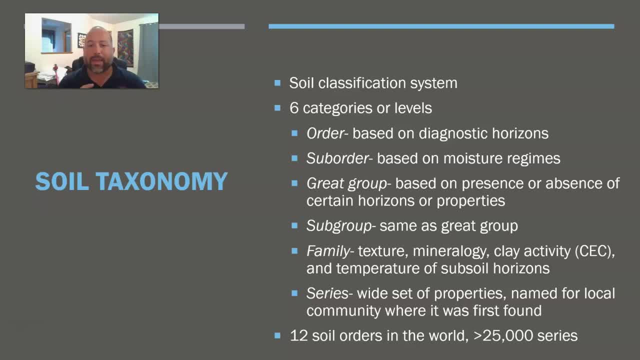 A property of the horizon that makes it this way And it's got a really strong evidence of that. Then we have sub order, which is going to be based on the soil moisture regime. We've got great group and subgroup, which are going to be based on the presence or absence of certain horizons or properties. 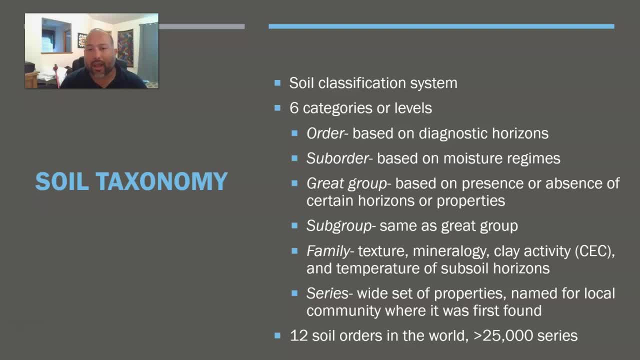 Then we have family based on texture, mineralogy, clay activity, where we're really talking about that cation exchange capacity, and then the soil temperature regime of subsoil horizons, And then we get all the way down to series, which is a wide set of properties. 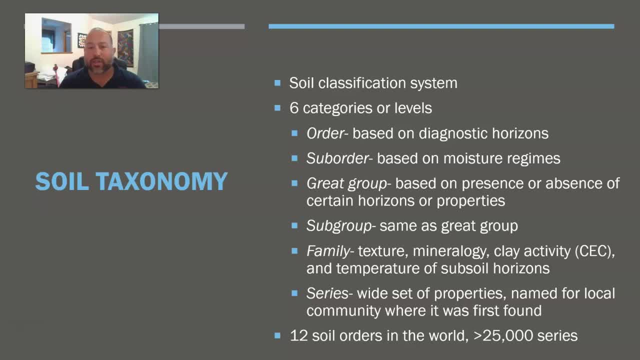 And it's going to be named for the local community where it was first described. So that's why you hear things like Bakersfield, Wasco, Granoso, Delano as series names. When we start at that highest level with order, we get down to just 12.. 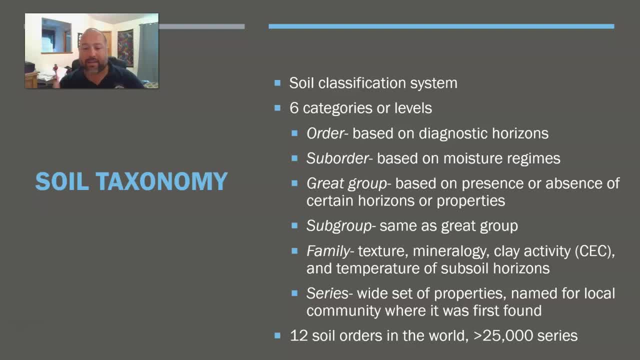 There's 12 soil orders in the whole world. When we're at the series level, there's over 25,000 series in the world. So it's we go from from very few categories- just 12 of them- to quite a wide array of categories, because soils can be so different in all the different places that you go. 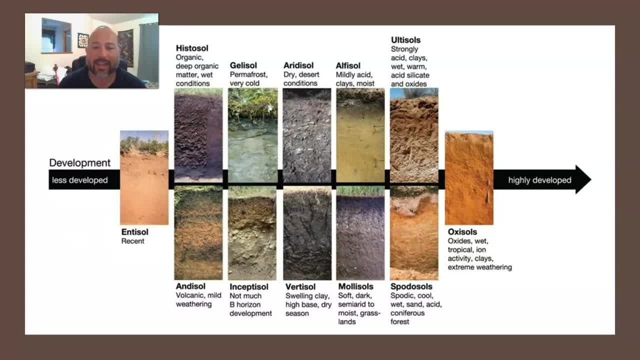 So here's a look at those 12 soil orders, and we will look at this again later on in this lecture. But just to give you an idea, we go from less developed soils to highly developed soils and we've got our 12 different orders there. 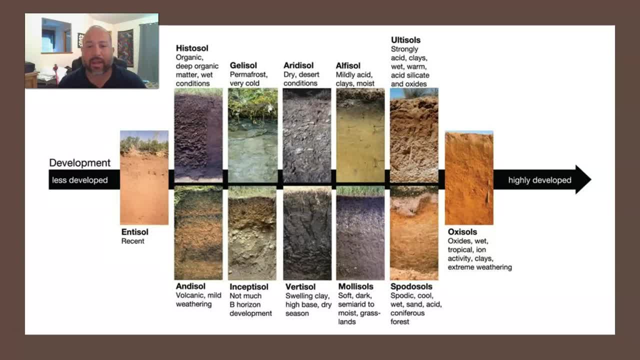 And you can see that they they look very different. but not only do they look very different, when you actually read through these descriptions they're pretty different. You go from something like an aridisol, where it says dry desert conditions, to a gelisol, which is permafrost conditions, to an inceptisol: not much bee horizon, andisol, volcanic, mild weathering, mollisol, soft, dark, semi-arid, moist grasslands. 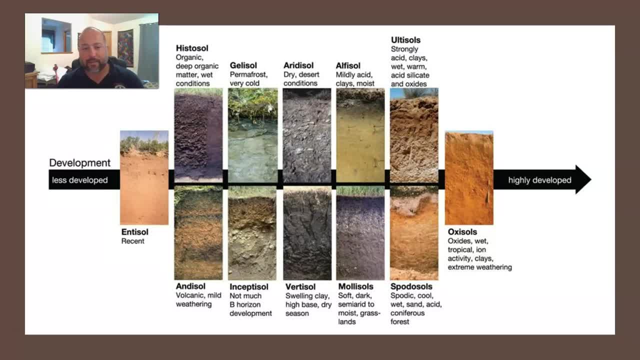 It's all very different. It's all easily, easy to understand, At least when we, Yeah, Think about it in this way, but it's not all it's. it's not always that way, right? The soil, soils don't just stay the same and they don't have just these perfect layers and it's just this soil all the time, right? 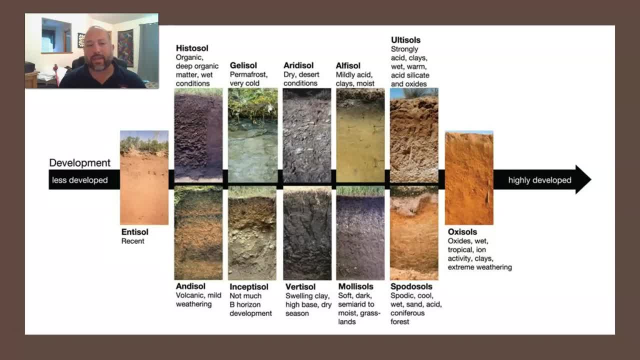 It's this layer, then it's another layer, then it's another layer, And so we get these mixtures. So we do our best to to try and classify all those soils and go get it down to the simplest of forms and orders. 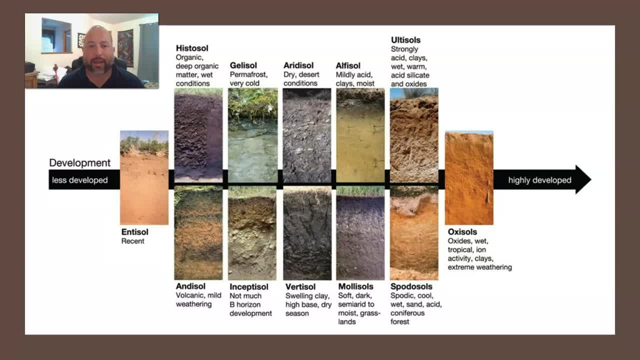 But then also, when we really want to know everything about The soil, we're down at that series level where we're going to have a big, long name attached to it, But that big, long name is going to tell us all the important properties of that soil. 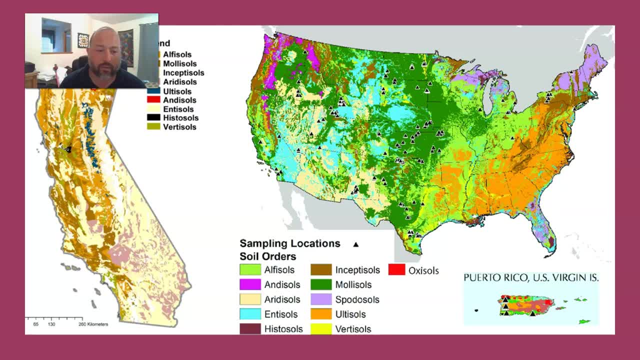 And so here's a look at both the nation and California, Bakersfield, where you know we're down there just north of the of the real southern part of the state and we actually will fall most of Bakersfield Falls into. 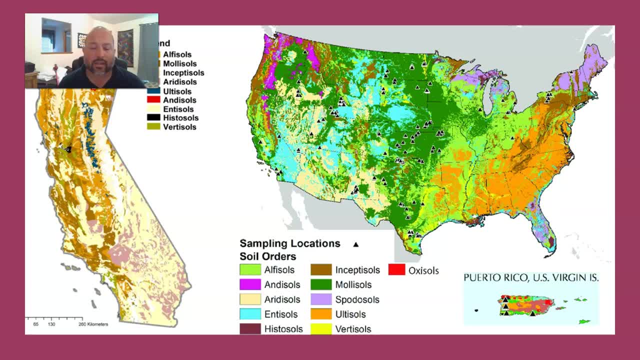 We have a temperature around 23 degrees Celsius. The, you know, transit some small hills around that western part of the state and you know we need some drought And then from there and then the you know we we have. you know that we've got the starting number of soil areas all over the state. 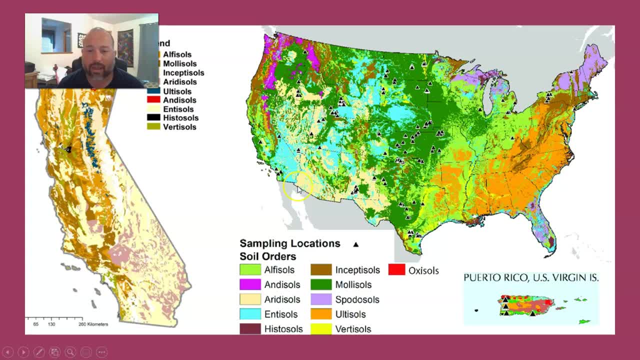 And you know it's just. this is the rapid rate, Or, um, you know, since this trees down. uh, how long have those fields been gone? I think the trees are dead to a picking up all these spine. 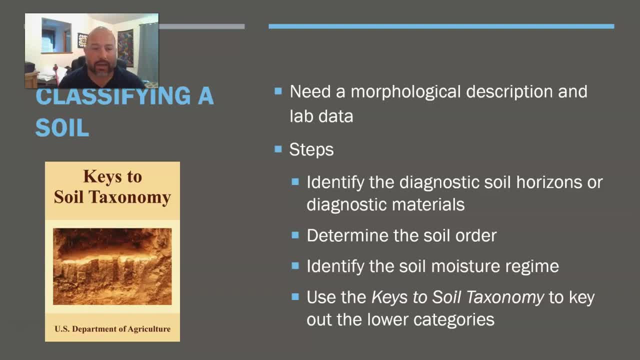 So, So this: how do you classify a soil? well, you're going to need a morphological description, which we learned how to do earlier. you'll probably need some lab data and then you're going to try and identify the diagnostic soil horizon, because if we figure out that diagnostic 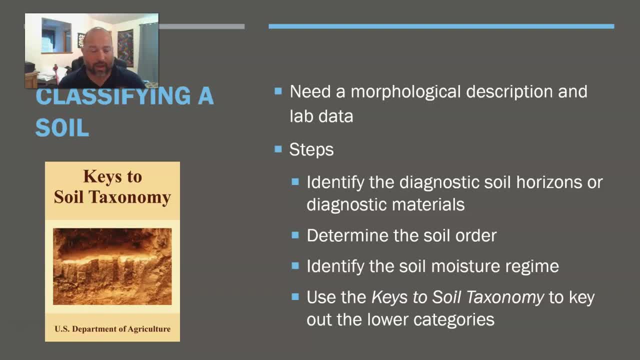 soil horizon. that gets us down to a 1 out of 12 um where we need to figure it out, and that's that's great, because if we can get down to figuring out, all right, which one of these 12 is it, that's much easier than which one of these 25 000 is it. uh, so once we figure out that diagnostic horizon, that 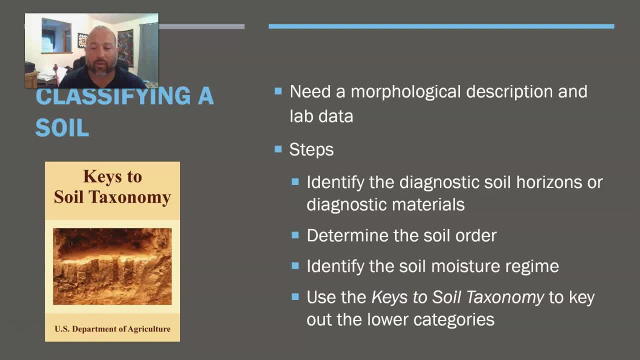 we can base our classification off of. then we'll figure out our soil order. then we can figure out our soil moisture is regime and when we figure that out that's going to tell us our sub order. and then we use the keys to soil taxonomy, which you can see a copy of right there we're going to. 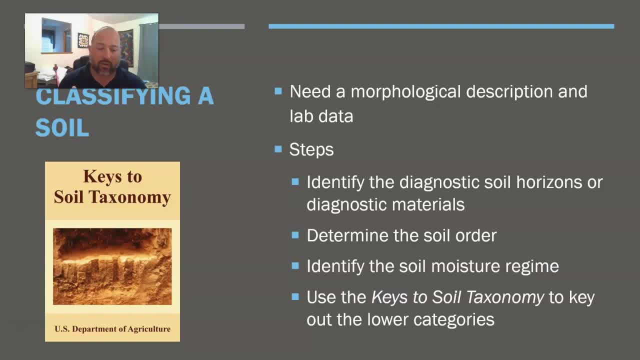 do that to key out the lower categories and figure out the, the great group and the subgroup and the and the family in the series and where we get down to all the way down to the series. and then we have all this nice information that tells us about what we want to know about that soil that we're looking at. 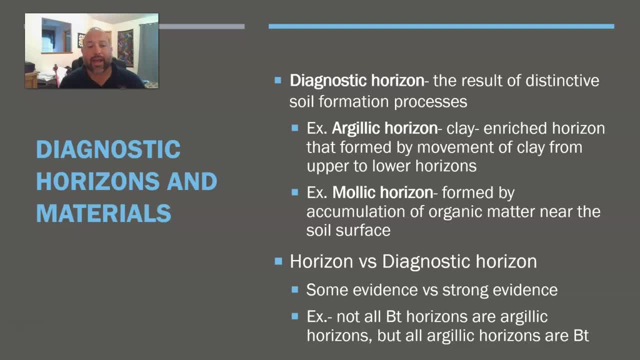 so i think the next question would have to be: what is a diagnostic horizon, and and how do we figure that out? because that's that's what we're saying. the first step in that process is: well, diagnostic horizon is the result of distinctive soil formation process, and what does that mean? it means 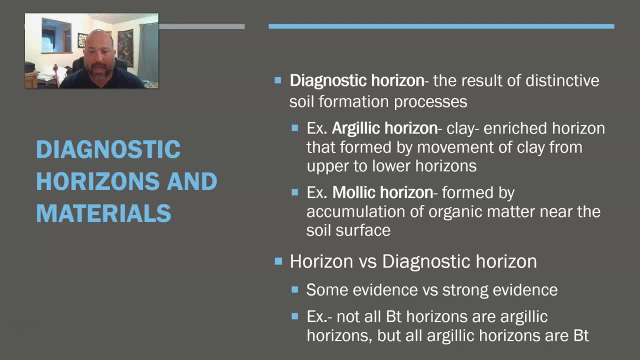 that it's something that is very obvious and it's, and it it's, it's very distinctive and compared to other ones. so the book gives two examples. it gives an argillic horizon, which is a clay enriched horizon, that formed by the movement of clay from upper to lower horizons. 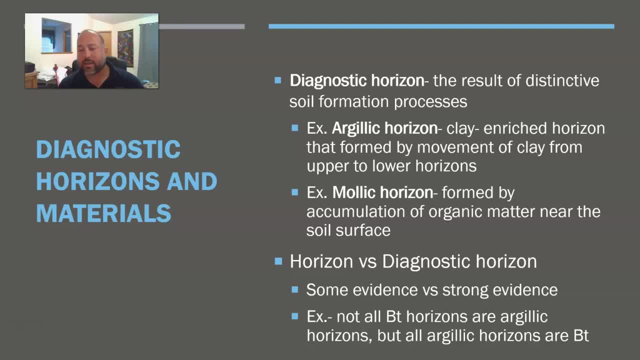 so that happens within certain soils. but then it also gives an example of a mollic horizon, which is formed by an accumulation of organic matter near the soil surface, and so mall mollisols are going to come from a mullock horizon, and because it they're formed by an accumulation of organic 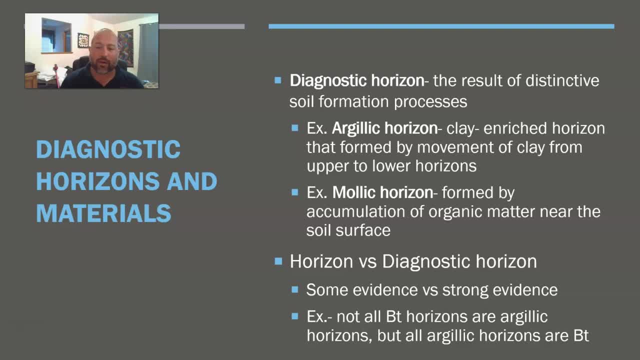 matter now tying in some of that knowledge we've got from before. that means those soils are going to be really dark. uh, clay enriched horizon, with the clay moving from um upper to lower layers, we're probably thinking: not, definitely not going to be as dark as a as a. 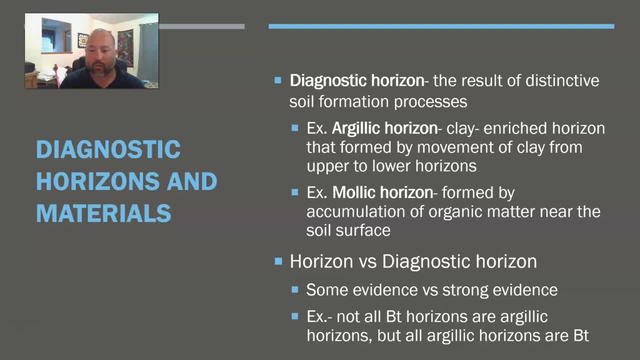 mollisol, because we're not talk. we're talking about clay, we're not talking about organic matter, but then if we're talking about clay, we're going to think about some of those properties, like we're going to think about the idea that it's probably going to hold water. really, 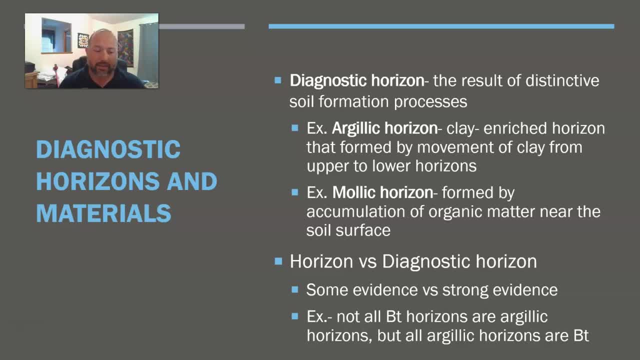 And it's not. it's going to have those sorts of properties to it that we think of. when we think of clay, as opposed to when we think of a mollusk on a mollusk horizon, we're not really thinking. well, what are we talking about? sand or silt? 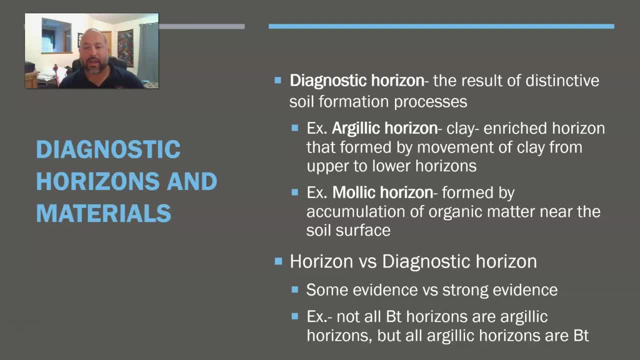 Well, with an argillic horizon, we're specifically talking about clay. So that kind of that really sends us off on, starts our thinking on: okay, well, we know this about this soil or we know this about this soil, and really kind of starts that idea of what's the important parts of this soil. 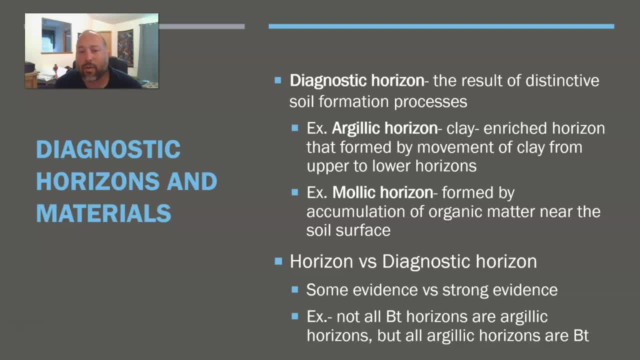 And then it's also important because we talked about horizons before. And so if you're sitting there going well, what's the difference between like when you classify a horizon from before Versus this idea of a diagnostic horizon? And the idea is the idea of some evidence of it versus strong evidence of it. And so if you take that first example, which is the argillic horizon from above, that would be classified as a BT horizon, right? 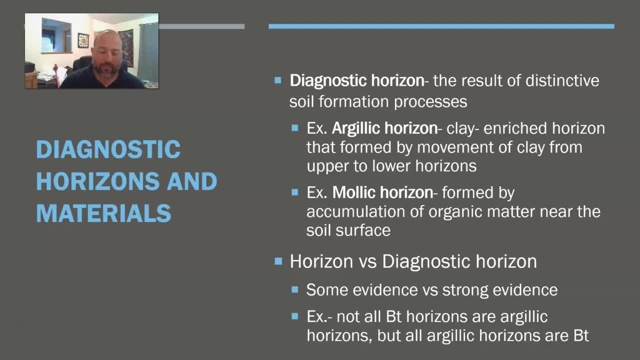 We'd see it in the in the subsoil, because we're talking about the idea that the clay moved from the upper to the lower levels. So we'd see it in the subsoil. So that's why it's a- B. 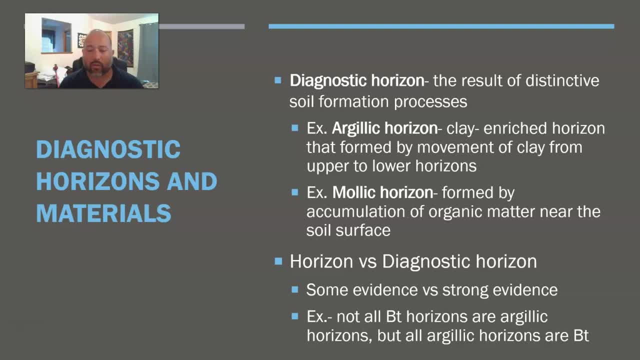 And then we'd see it in the subsoil, So that's why it's a B. And then we'd see it in the subsoil, So that's why it's a B. And then the lowercase T is that idea of an argillic horizon. But now the difference between that, what just any BT horizon, versus an actual diagnostic horizon, is that it's got to have strong evidence that this is the overwhelming thing that's happening, not just that there might be a little bit of it happening. 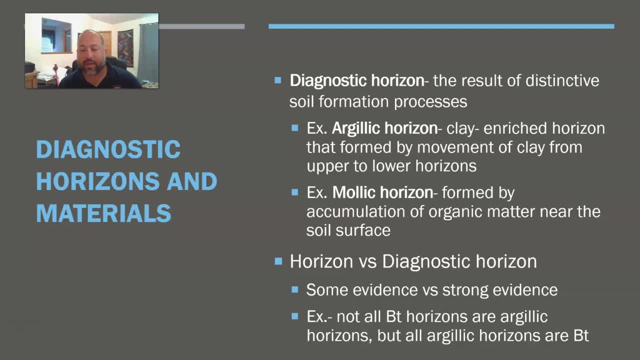 So it's the idea of some evidence versus strong evidence. So not all BT horizons are considered argillic horizons that this diagnoses. But anything that is an argillic horizon, anything that is a diagnostic horizon, would definitely be classified as BT. 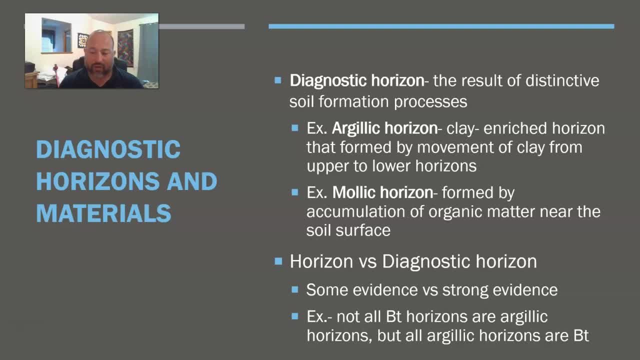 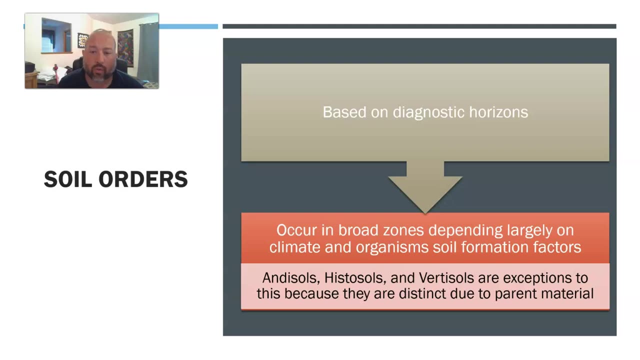 And so it's just the idea that that it has to have strong evidence that this is the definite soil formation, this distinctive soil formation process that's happening right here, And so when we go then to determine our soil order, that's based on our diagnostic horizon. 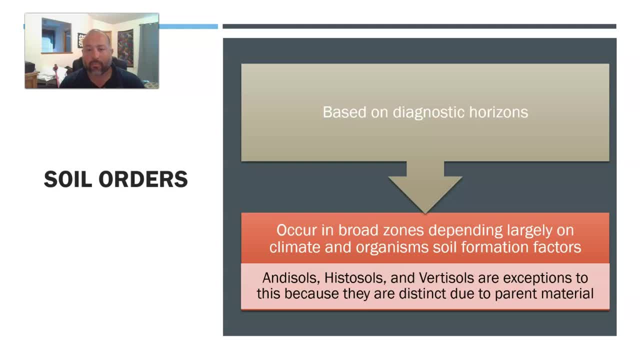 And soil orders are going to occur in broad zones, like we looked at the map of the US and saw kind of how broad some of these zones can be, And it's going to depend largely on the climate and organisms when we think about our five factors of soil formation. 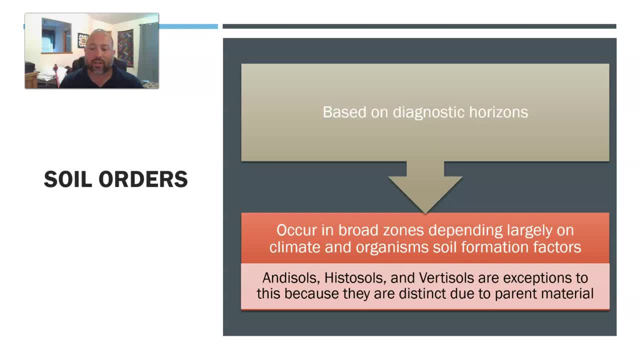 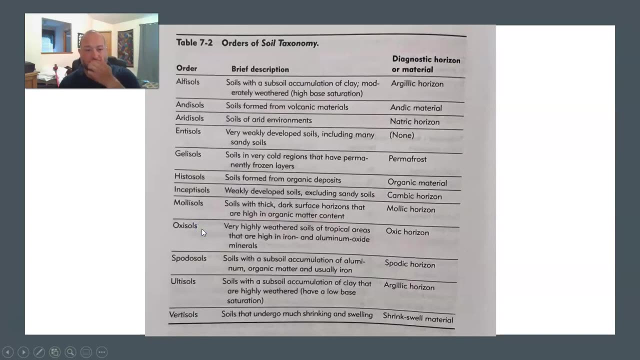 Andesols, histosols and vertisols. those three out of the 12 soil orders are actually different because they depend more on the parent material soil formation factor instead of the soil formation factor. So let's look at those 12 soil orders, with a brief description and the diagnostic horizon that makes it so. 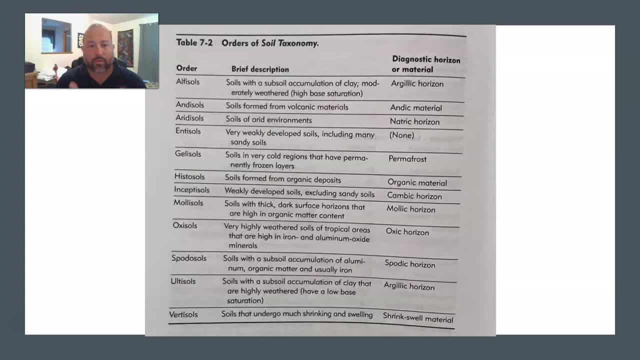 And so we talked about argillic horizons, and so that would lead us to alphasols, and it says soils with a subsoil accumulation of clay moderately weathered, Which makes sense because we know if you have an argillic horizon, an argillic horizon has that evidence of the 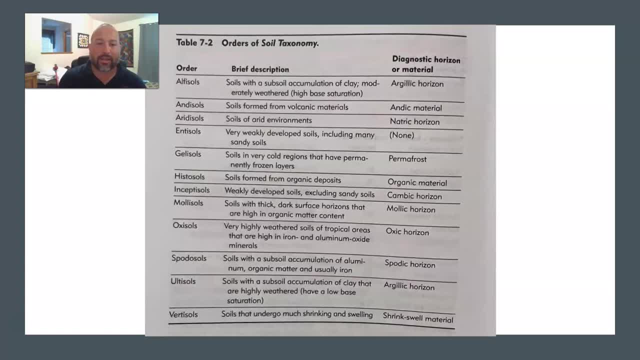 Clay moving from the upper to the lower levels. so then the idea that alphasols have a subsoil with an accumulation of clay. that makes sense. And now that tells us a whole lot about what's going on already, and we can start getting a picture of, maybe, what that's going to look like in our head if we, you know, dig a soil pit and look at that soil. 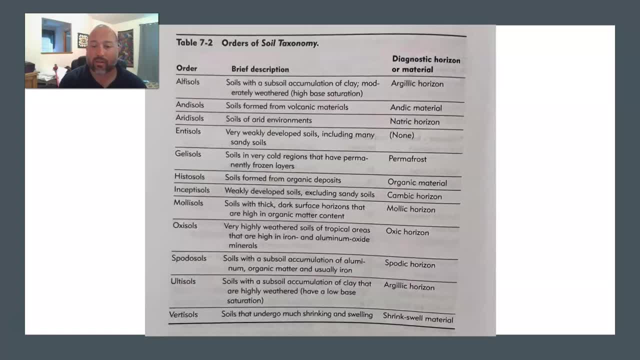 Whereas something like we'll see around here eridisols. it says soils of arid environments and then it says A nitric horizon, and so nitric is similar to argillic and it's going to have that similar idea of the subsoil accumulation of clay, but then it also has the idea built in of it that it's got a specific structure to the soil. 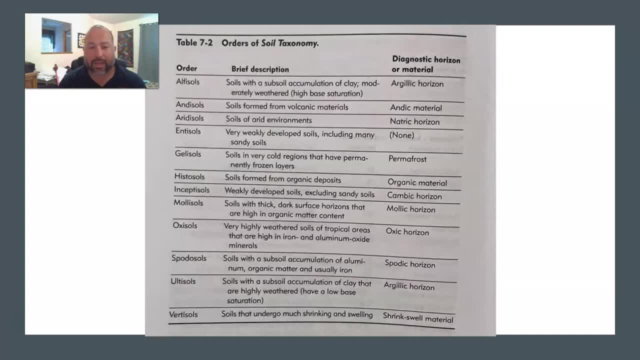 It's got that columnar or prismatic or blocky type of soil to it and then also, specifically with the cation exchange Capacity, it's got high amount of exchangeable sodium, and so there's all sorts of different reasons as to how these things form with something like the gelisols. 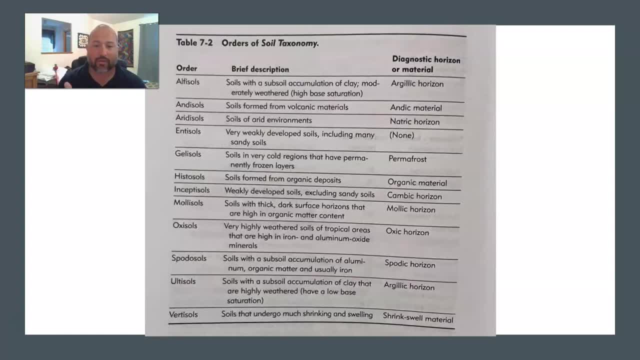 It's. the diagnostic horizon is permafrost, so anything that's a gelisol is going to be soils in very cold regions, that are regions that have permanently frozen layers With mollisols- we talked about that earlier- before that mollic horizon, that thick, dark soil. 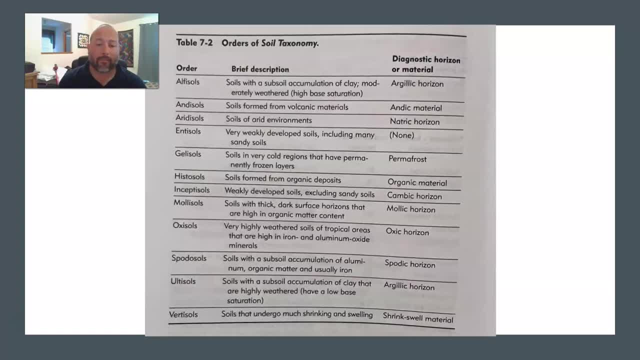 It's a surface horizon that's going to be full of organic matter, That's going to end up as a mollisol, and so it just depends on where you go and what you've got going on, because you can see even something when you go down to an ultasol. that's also an argillic horizon and you're like, but it's got to be something distinct. 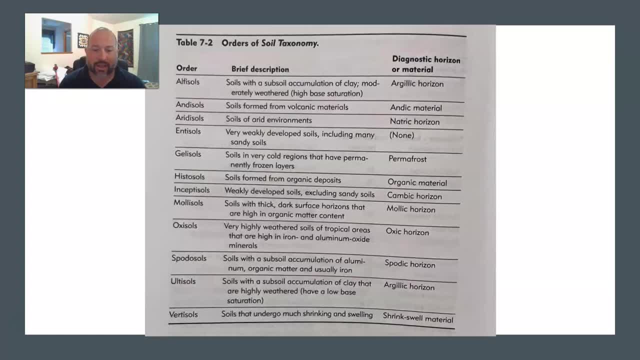 But then you read and it says: soils with a subsoil accumulation of clay that are highly weathered. so they also have that accumulation of clay, but they're just older soils that have been weathered quite a lot, Whereas the alphasols are going to be a little bit younger soils. and so once you start getting used to these terms, you can really start. even though these words seem like they're complicated, they tell you a lot about what you're looking at and what you're dealing with already. 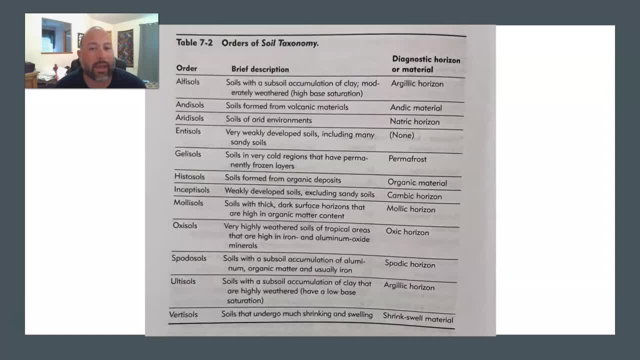 And then you know, you can look at it at the way of you're trying to figure out what's happening with your soils. so you need to figure this out. but then also let's look at it the other way, because a lot of this work has already been done. 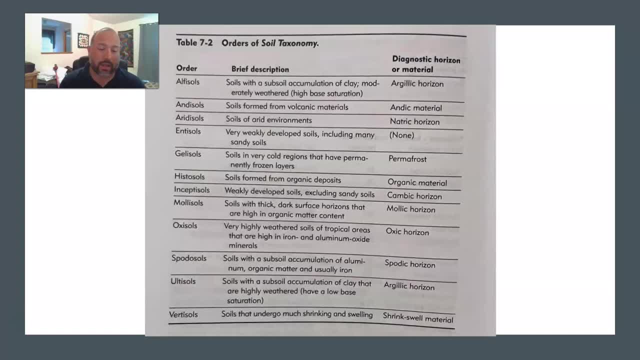 For us already. so really, what we're doing is, you know, we're clicking on an area in some sort of a mapping, a soil mapping app, whether we're using SoilWeb or WebSoilSurvey or something else- and all this information is already available to us. 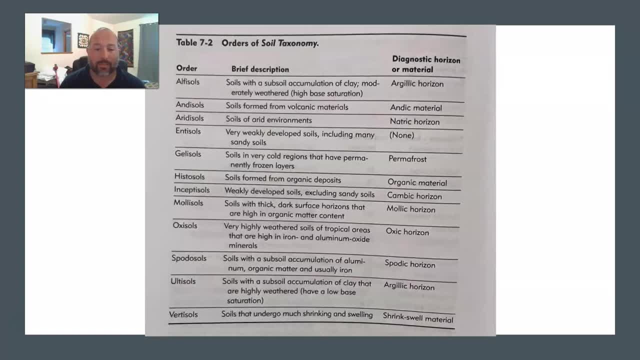 We just have to be able to read it and understand what it means. when we see that it gives us this whole long name and we're like: well, what does that mean? Well, it tells us a whole lot about that soil. We just have to be able to. 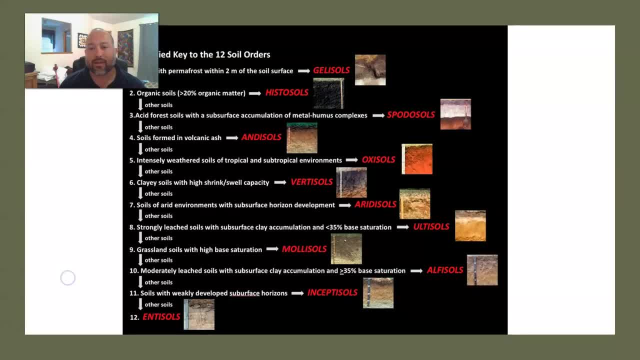 To put together the pieces, so to speak. So here's a simplified key, another way to look at it, to where you can start off with number one here and then work your way down. So if you have soils with permafrost, oh well, my soils aren't permafrost. 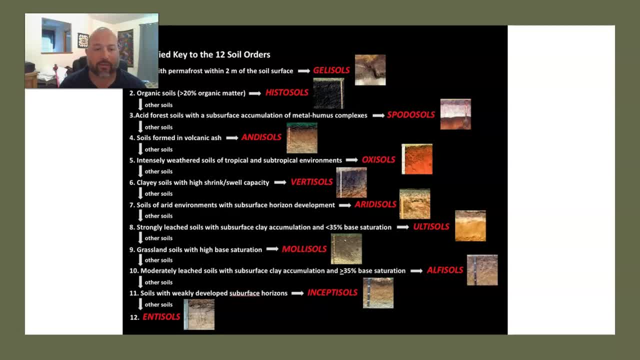 Okay, well, do your soils have a ton of organic matter? No, they don't have a ton of organic matter. Okay, keep going. Acidic forest soils: well, they're not in. there's not a lot of forest here. 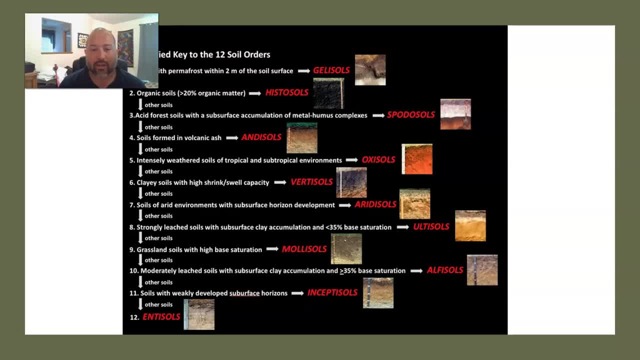 Okay, well, it's not that soil's formed In volcanic ash? well, no, that's not really us either. Intensely weathered soils of tropical and subtropical environments- well, we don't have a tropical environment. Keep going. 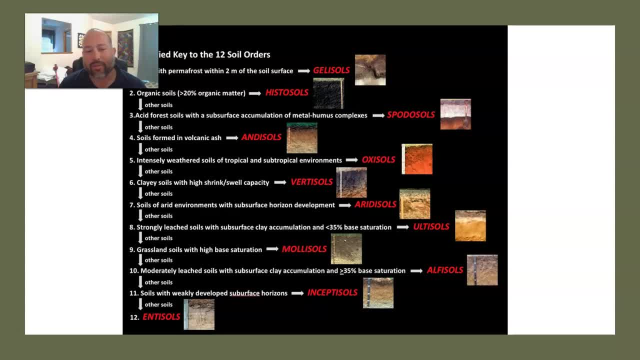 Clay soils with a high shrink soil capacity- no, we don't really have that either. Soils of arid environments with subsurface horizon development: we got that- Iridosols. look at that boom and we stop, And so that's a. it's a super simplified key, but it's a nice easy way to kind of figure out what it is you're dealing with and a quick way to get there. 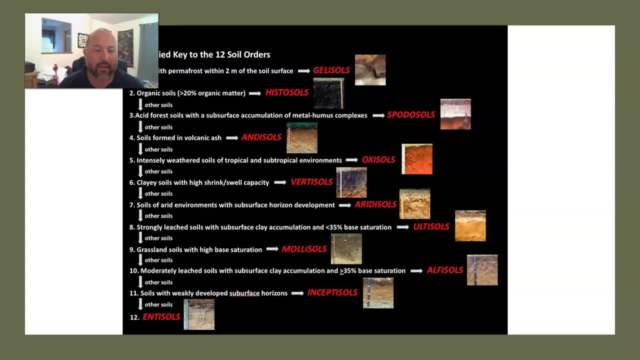 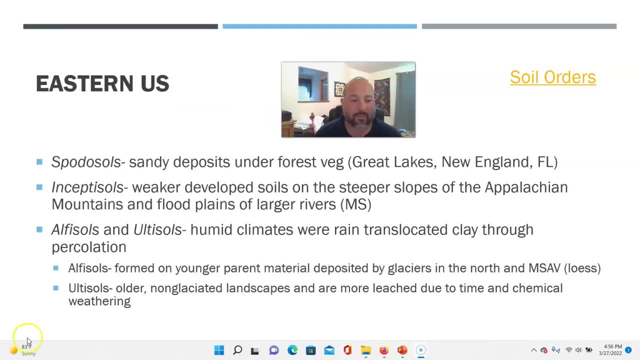 And once we figure out the soil order, we can start putting together the other pieces as well. So when we're talking about the oops, there you go. Made myself disappear for a second, but I'm back. So with what we just talked about in terms of the soil orders, right here on the upper right. I've posted a link here to the University of Idaho. 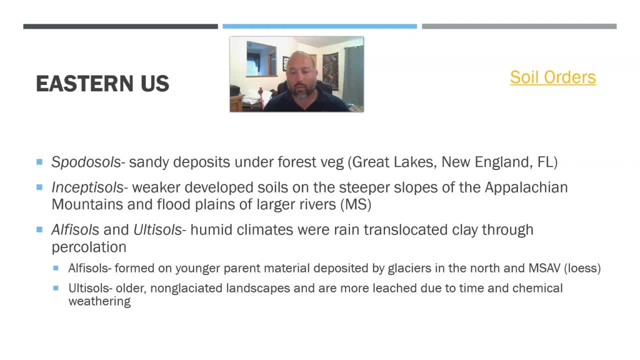 and they've got a very descriptive website set up to Really dig into the 12 soil orders and show you pictures of it and give you a big long descriptions of it. So if you want to pause the video right now and click on that link and check, check out those, those 12 soil orders, go ahead. 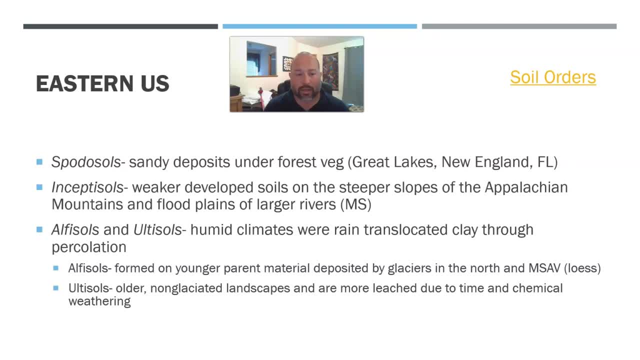 And so breaking it down in terms of where are these soil orders and what really are they. So in the Eastern United States you got spodosols, enceptosols, alphasols and ultasols. With spodosols, you're talking about sandy deposits. 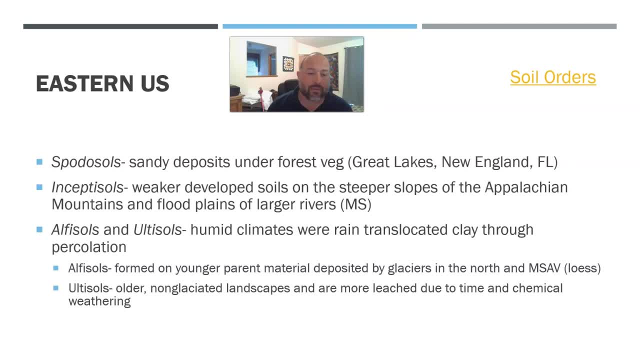 Okay, It's under forest vegetation. So it's the Great Lakes areas, New England and Florida. Your enceptosols are going to be weaker. developed soils on the steeper slopes of the Appalachian Mountains and floodplains of larger rivers like the Mississippi. 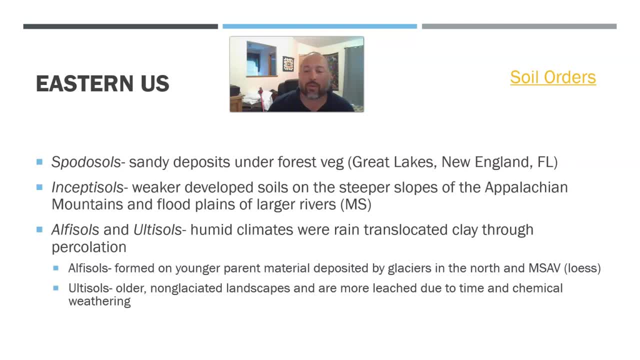 Your alphasols and ultasols are going to be in humid climates where rain translocates the clay through percolation and gets you that clay going from the upper levels to the lower levels Because, remember, both of those have argillic horizons, which is that clay moving from the upper level to the lower level. 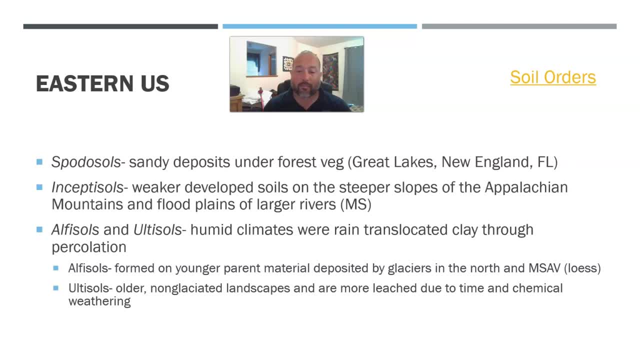 Your alphasols. Your alphasols are going to be formed on younger parent material that were deposited by the glaciers when that happened. You're also going to see alphasols in the Mississippi Alluvial Valley. So I've mentioned this before. but if you ever have gone down to the Mississippi Alluvial Valley, you're supposed to be going down and down, and down. 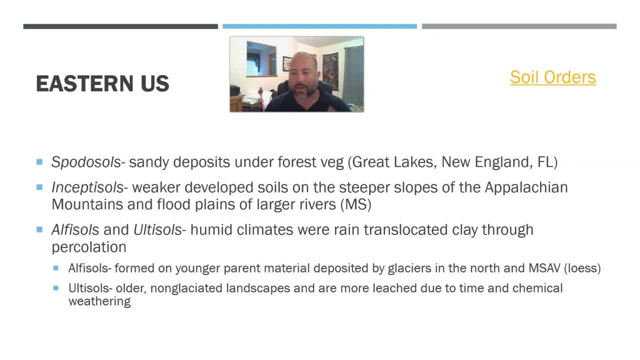 And then all of a sudden, you kind of hit these hills and you're like, where are these hills come from? And what it is is it's all this silt getting deposited Down the river And you end up with these hills and, through wind erosion and water erosion, just bringing all this material and ends up forming these hills. 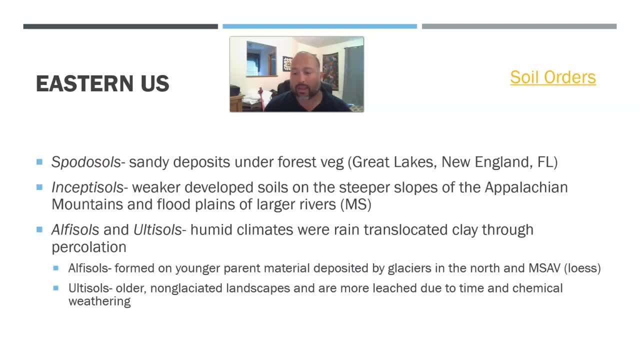 And those hills are called lusts And that's how the Mississippi Alluvial Valley formed, And so you're going to find that's where you'd find alphasols- That's one area specifically- Whereas ultasols older 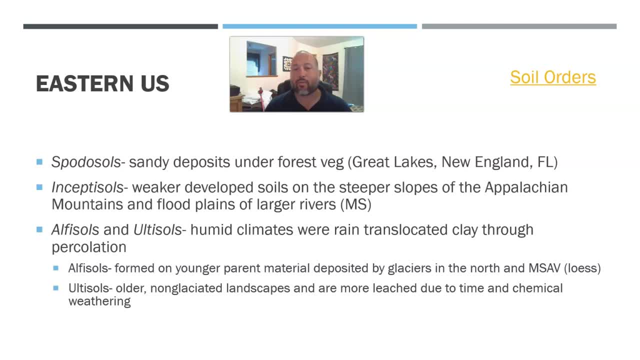 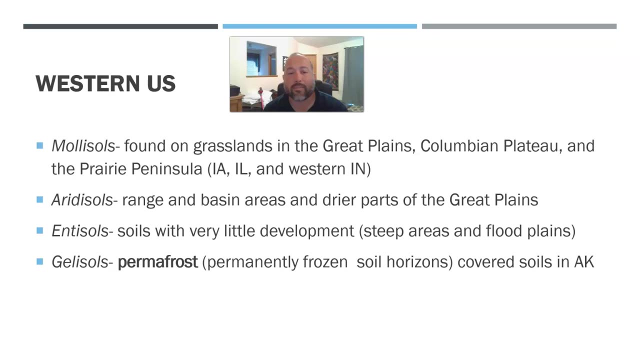 Non-glaciated landscapes. they're more leached due to time and chemical weathering. So really, your older landscapes before everything was frozen over and all that. those ones are going to be ultasols. In the western US you've got your mollusols, which are going to be found on grasslands in the Great Plains, the Columbian Plateau and the Prairie Peninsula. 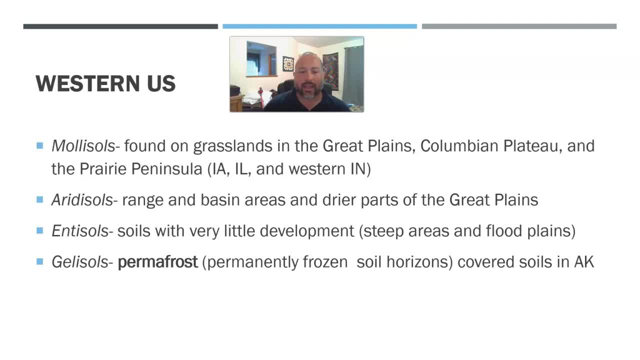 Which is a stretch from Iowa, Illinois and western Indiana where the Great Plains kind of extends, And so that's remember, mollusols are going to have that higher organic content, Really dark soils, Erythrosols, your range and basin areas in the drier parts of the Great Plains, as well as, of course, the drier parts of the Central Valley as well, because that's what we have here. 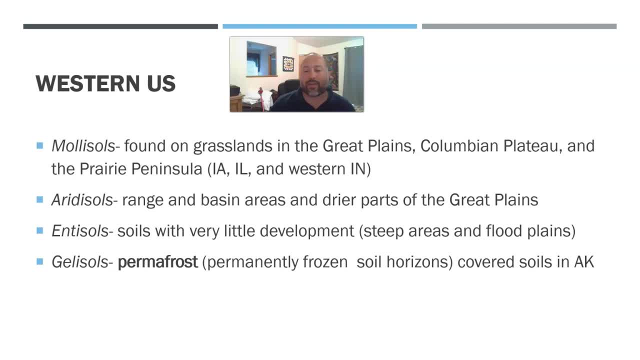 Your entosols are soils with very little development. So you're going to find that in steep areas and floodplains or areas where you get a lot of erosion, because the soil keeps moving and moving and moving And that's why you have soils with very little development. 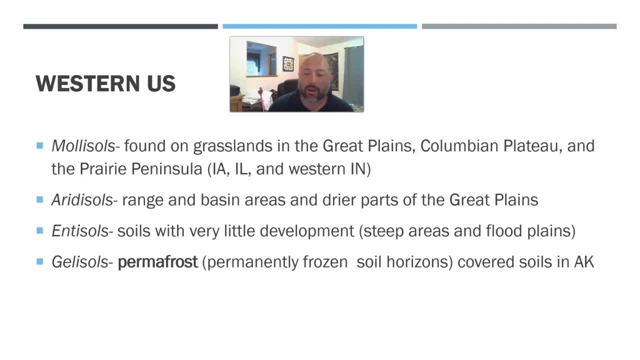 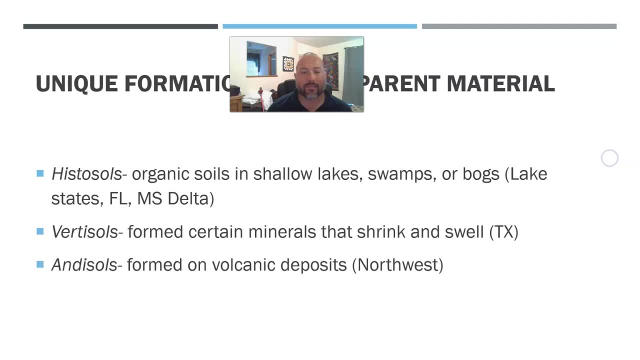 And then our gelosols, which are permafrost, which are going to be permanently frozen soil horizons- That's how we define permafrost- And we're going to see those mostly in Alaska. Let's slide myself over here. 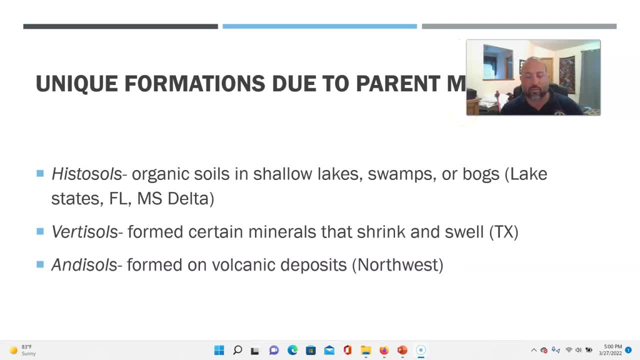 So unique formations due to parent materials. We said there were three soils that didn't really go with the idea of specific climate and organisms. It was more based on their parent material, So that's histosols, which are organic soils in shallow lakes and swamps. 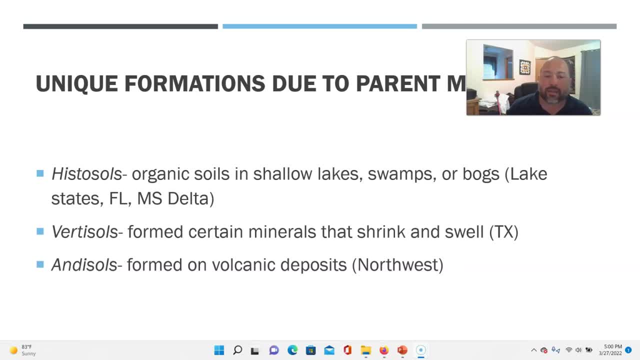 So the lake states, so the Great Lakes area, the Florida and the Mississippi Delta. you'll find some histosols- Your vertisols are flora- And you'll find some histosols in the Mississippi Delta, Formed with certain minerals that shrink and swell. 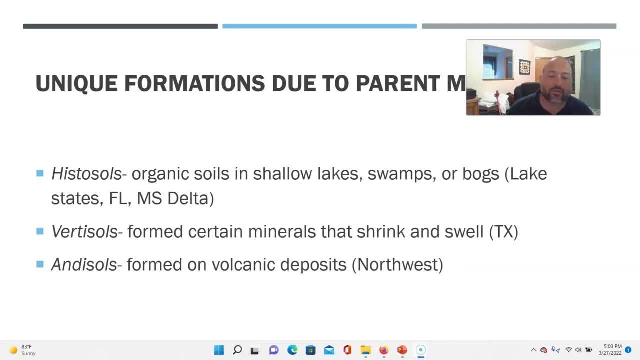 And you're going to see that a lot in Texas. And then your andesols, which are formed on volcanic deposits, So you can see that a lot in the Pacific Northwest. Think like Mount St Helens, Mount Lassen area for those of us in California. 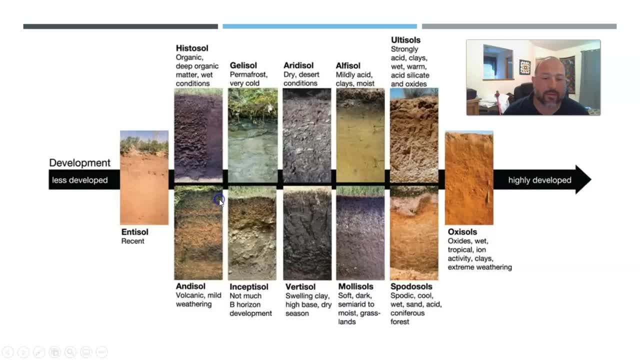 Those areas are going to have andesols, And so we're back here again with these 12 soil orders And really just kind of hopefully Having this make a little more sense, This idea of less developed soils to more highly developed soils. 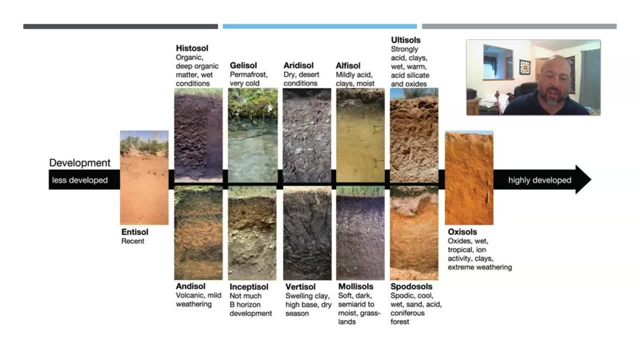 And really we can even think about the idea of younger soils versus just way older soils And soils that have been really, really weathered, That's that highly developed versus the less highly developed, And so you can just see where these different soils come into play. 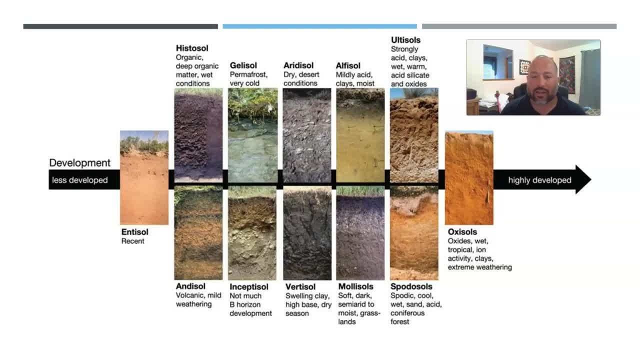 So our iridesols that we have here, Dry desert, Dry desert conditions that kind of make sense for Bakersfield When you really think about it versus some of these other areas And when I look at the soil in my yard, Just looking at this picture and thinking about the iridesols. 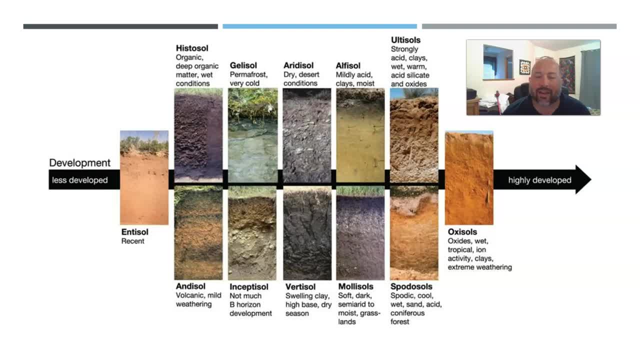 I'm like, yeah, I can kind of see it, But you know, not everywhere is going to give you that perfect lining up And the idea of soils changing and having all the different layers In between. not everything is going to look perfectly the way it does on this picture. 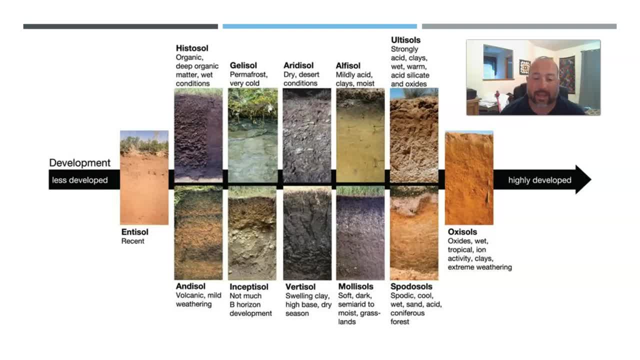 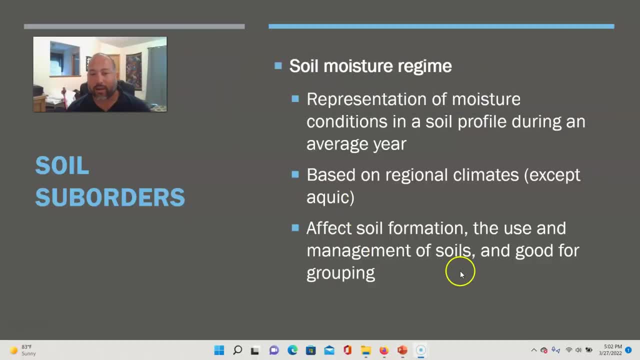 Yet you might still have. it still come from the same order. So, in terms of our sub orders, I'm going to slide myself back over here again. So sub orders are going to be based on your soil moisture regime, which is going to be a representation of moisture conditions in a soil profile during an average year. 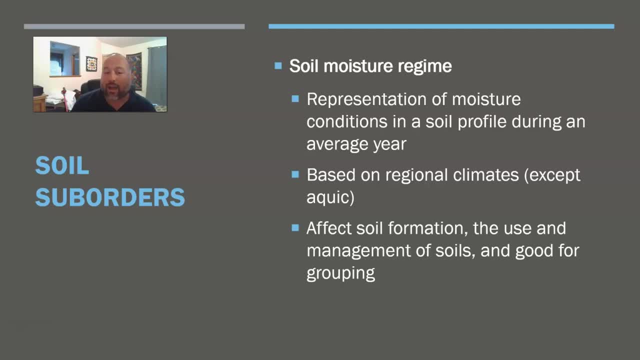 It's going to be based on your regional climates, except if it's an aquic. So it's going to be based on the soil sub order and your soil moisture regime really affects your soil formation, the use and management of the soils. and it's good for. it's good for grouping, because it's really easy for us to come up with just a few categories to make it make sense. 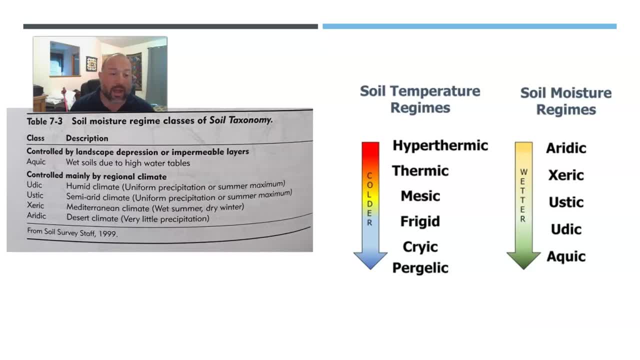 And so, if we look at the categories, we've got aquic. That's the one that we said isn't going to be dictated by climate. What it's dictated by is high water tables. It's controlled by landscape depression or impermeable layers. 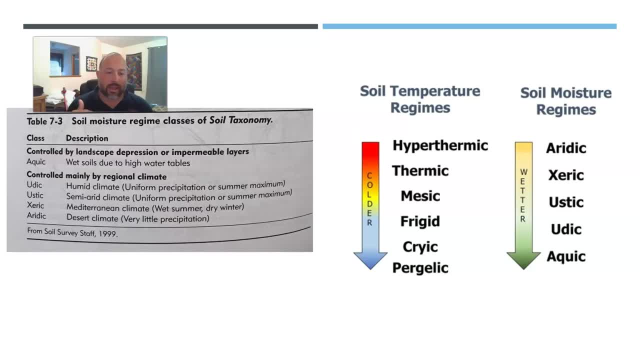 So you got either Depression, where the land's low, that the water tables high, or the idea that you, that you have impermeable layers. The other ones are going to be controlled by climate. So Utik is humid climates, Ustik semi-arid climates, Zirik is a Mediterranean climate and Eridik is a desert climate. 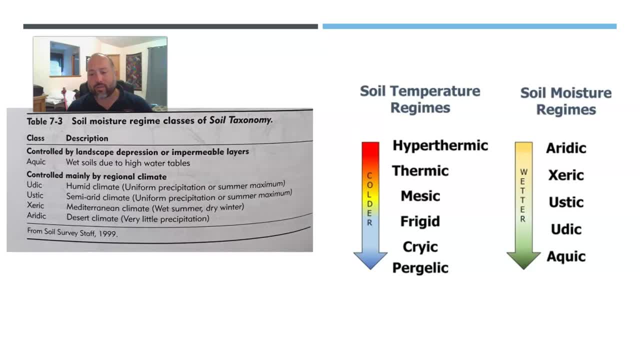 So we're going to see these terms come up when we get to the idea of the, of the sub order, Also here On the right, So you can see our sub orders, or our sub orders, or our soil moisture regimes, whichever way you want to think about it, going from drier to wetter. 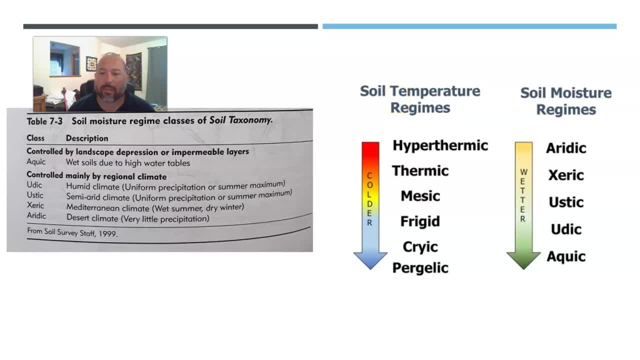 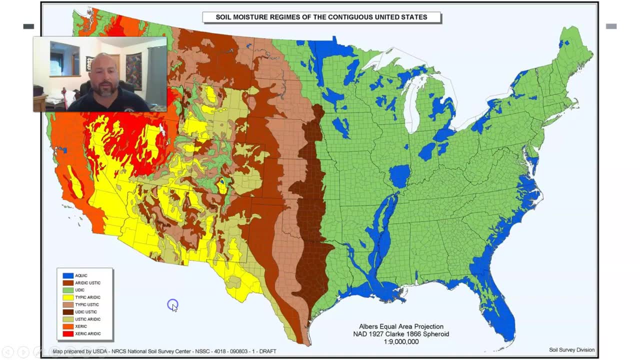 And then also- we'll see this later on when we're talking about families- But soil temperature regimes, the idea of going from hotter to colder, And so here's a look at our soil moisture regimes So you can see we get kind of typical eridik out here. 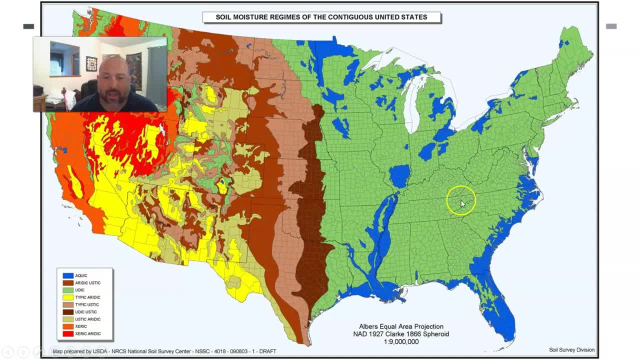 And in Bakersfield, as opposed to something like Utik for a lot of the eastern United States or the Aquic, these Aquic areas which makes sense for the for the eastern United States right on the, on the borders and on the Mississippi Valley area here. 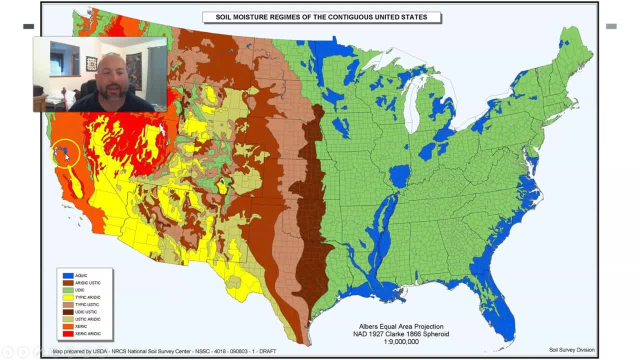 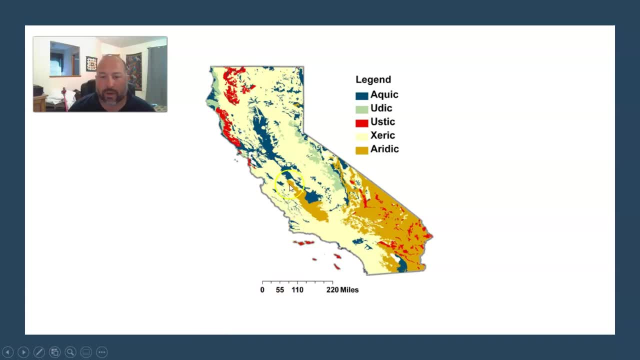 You can also see that Aquic area for our San Francisco Bay areas, our Delta areas up in the upper part of the Central Valley. So Okay, So in California- here's a more close-up look at California- We've got our aquic areas, which are the delta areas. 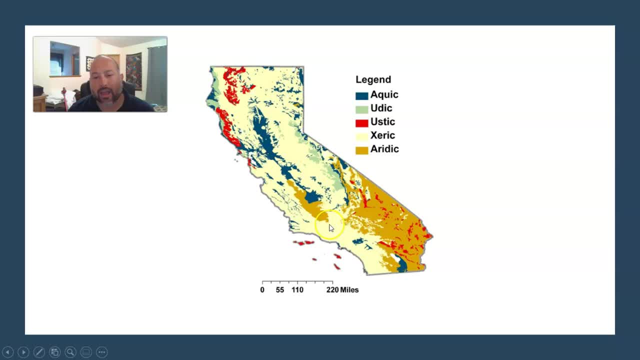 And then you can see udic ustic And you can see they classify us more xeric, but you know xeric aridic. I think it kind of depends on exactly where you would fall on this map, But those you know really dry conditions. 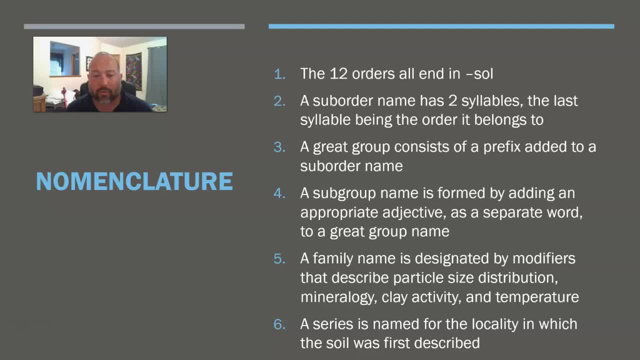 So in terms of the nomenclature, so trying to really understand the words that we're going to see when we're seeing the description of the soil classification, the whole soil taxonomic name or taxonomic classification- a few rules to kind of remember. 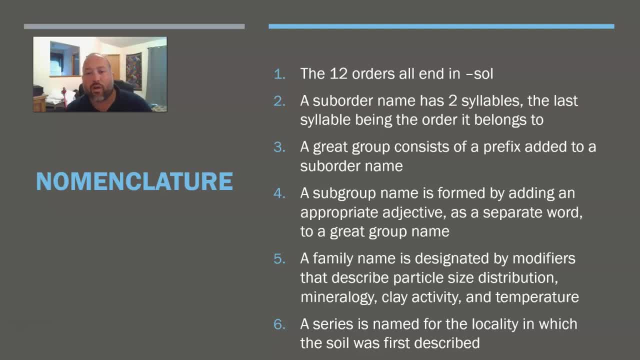 Bam got him. The 12 orders all end in sol. S-O-L There is. Depending on where you're at, it might get a little more complicated than that, But the 12 specific soil orders do all end in sol. 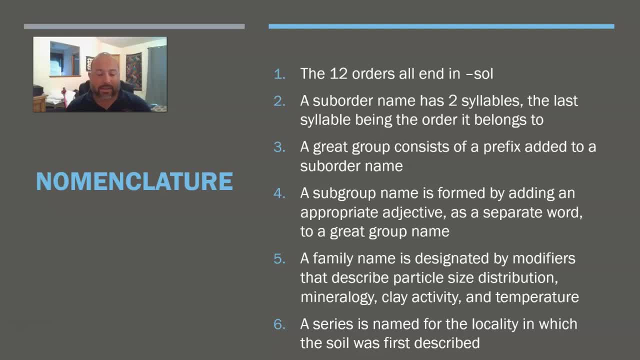 Now you might get something where the name doesn't end in that typical soil order, but you can figure out which soil order it does fall into with a little bit of Googling or just a little bit of extra knowledge. A suborder is going to have two syllables. 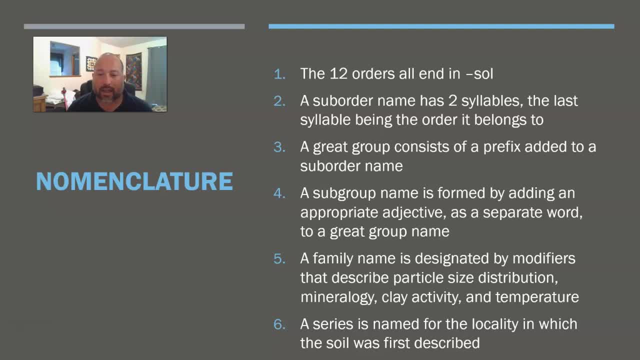 and the last syllable is going to belong to the order that it belongs to, So it's going to have Part of the order name within the last syllable. A great group is going to consist of a prefix added to a suborder name. 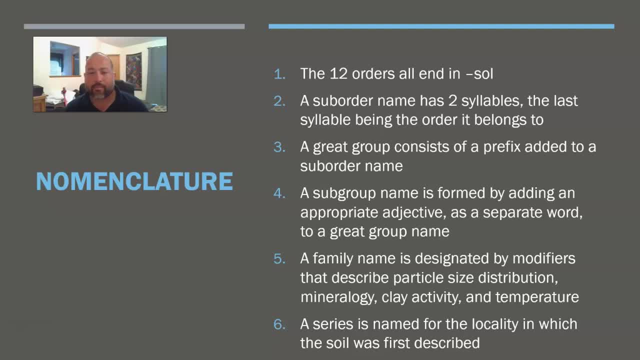 So there's going to be a prefix and then the suborder name, And then a subgroup is formed by adding an adjective as a separate word to the great group name, And then a family name is designated by modifiers that are going to describe the particle size distribution. 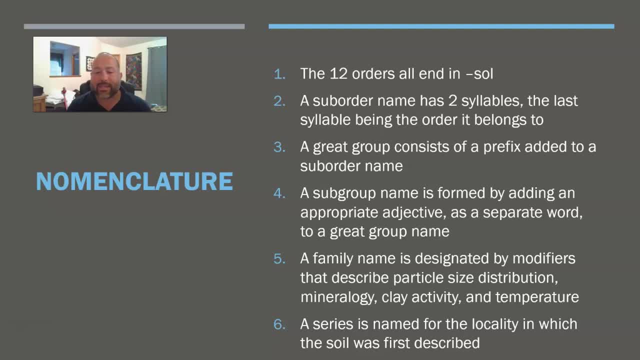 the mineralogy, the clay activity, which you said was that CEC, the cation exchange capacity, And then And then the temperature, And then the series name you said is going to be named for the locality in which the soil was first described. 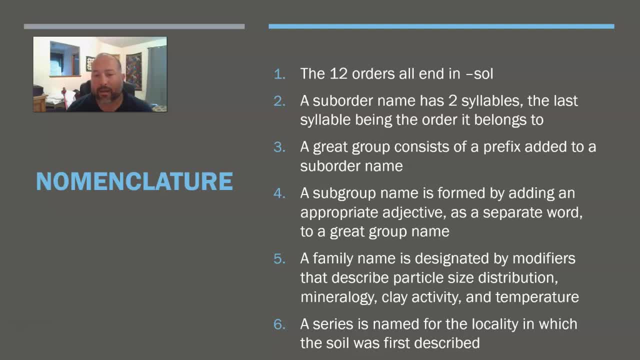 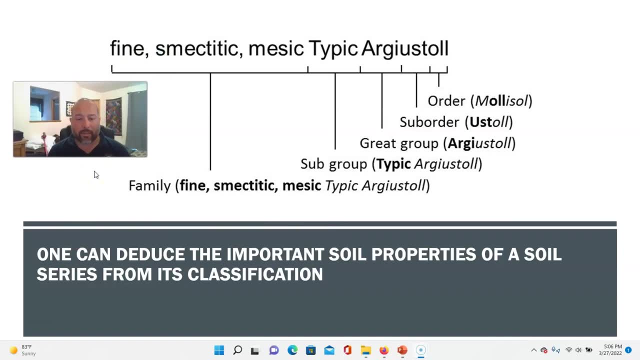 Does that totally make sense to you? Maybe not, but let's kind of put it together. So let me just move myself out of the way so you can see this clearly. So here is an example, And we want to also go over the idea that we can figure out the important soil properties from the name. 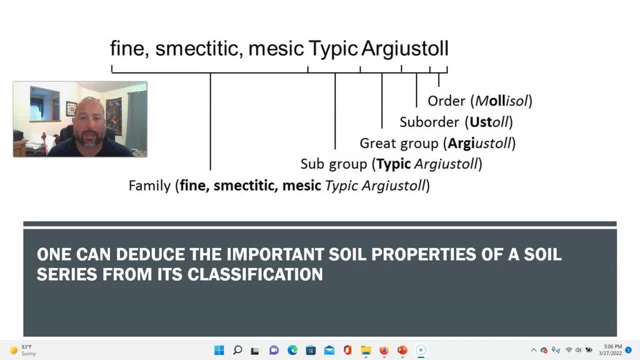 So if the name is fine- smectitic, mesictipic, RGU- we're saying they're going. what does that mean? But we have actually learned about all this stuff. So mollisol is our order And because we see this all within the name there, that's how we get our suborder or our order. 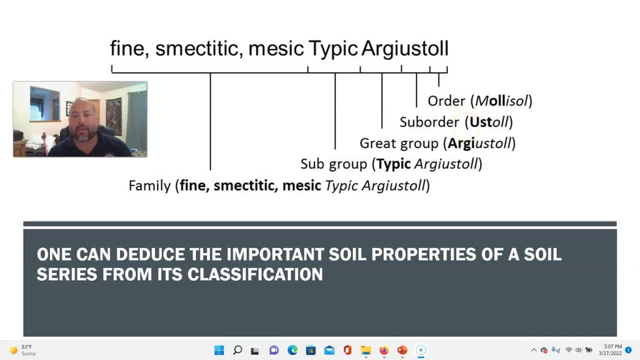 Our suborder is our ustol, which we said. that idea of the order would be the Okay Okay, Okay, Okay, Okay, Okay, Okay, The last syllable in that two-syllable name. So we've got ustol. 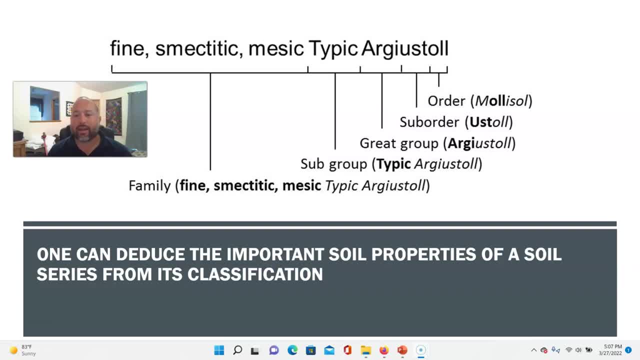 So that ol takes us back to our order, Right, And so now our great group is our RGUstol And our subgroup is our typic RGUstol, And then our family fine, smectitic, mesictipic RGUstol. 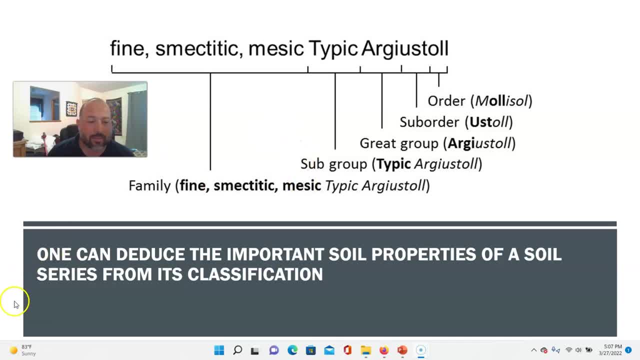 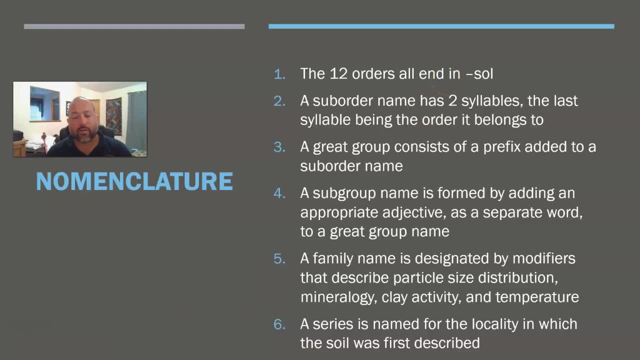 So now I'm going to go back a slide here because I really want you guys to get this idea. So now remember, the 12 orders all end in sol. so we figured out, we had our, our oll. that tells us: it's a, it's a mollisol, and 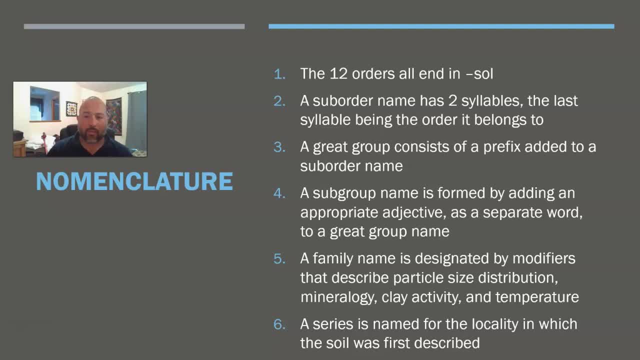 mollisol ends in sol, a sub order, right? so let's go forward here. so our sub order is ustal, right? so a sub order name has two syllables, the last syllable being the order that it belongs to, so that oll that tells us it's a mollisol, and then the ust tells us um, tells us the, the soil moisture. 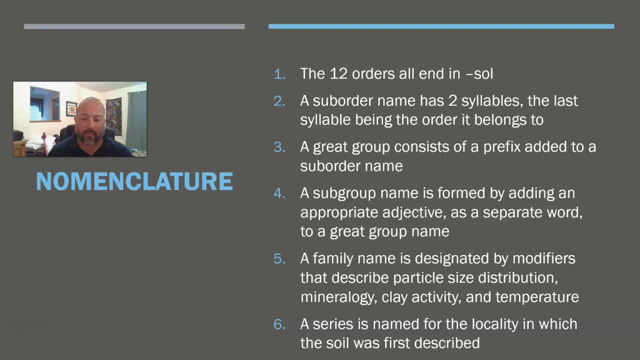 regime, which is ustic, which is um, tells us it's the idea, the idea of a semi-arid climate. and so we've got it's a. it's a mollisol. so we know, now trying to add that important soil properties to it. so it's a mollisol. so we know it's probably a grassland area. we know that it's going to have. 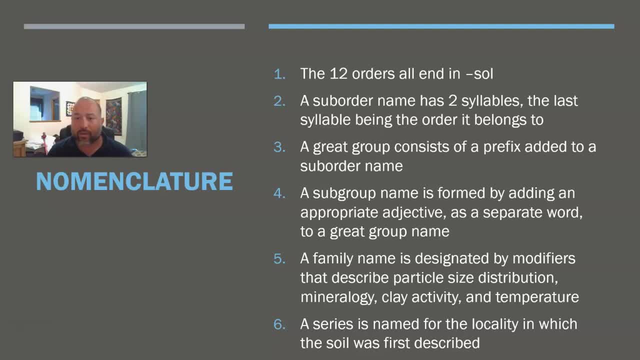 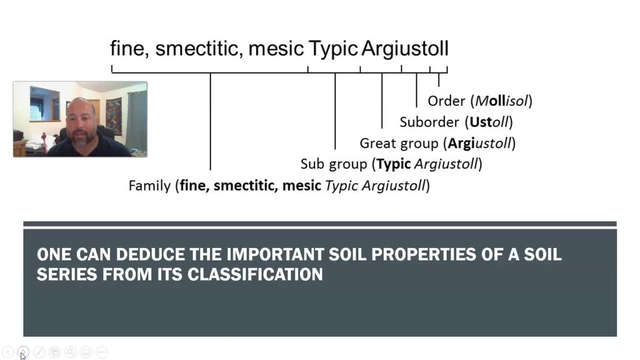 a heavy amount of organic matter. it's going to be a dark looking soil and it's going to be a semi-arid climate. so that's what we've figured out so far just by looking at the name. now let's go back to the great group rg ustal. so now being that we kind of talked about that. 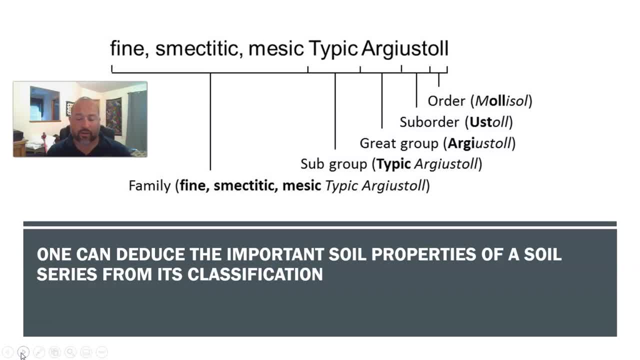 earlier. we know the idea of rg means that there's an argillic horizon there, which is that idea that it's got the um, the clay, moving from um, from upper to lower levels. so we know it's a, it's probably a grassland soil, heavy organic matter content. it's semi-arid climate. 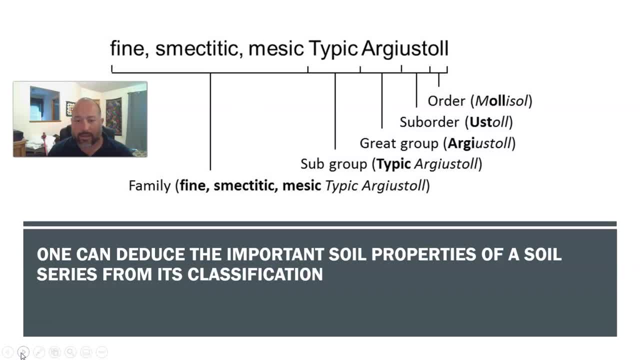 it's got an argillic horizon typic, so it's um, so it's going to be typical of what we would expect. and then we get down to the family. so fine, so what? the? our particle size is fine, so, um, where we think about our, our particles in terms of, um, our fine medium grain. 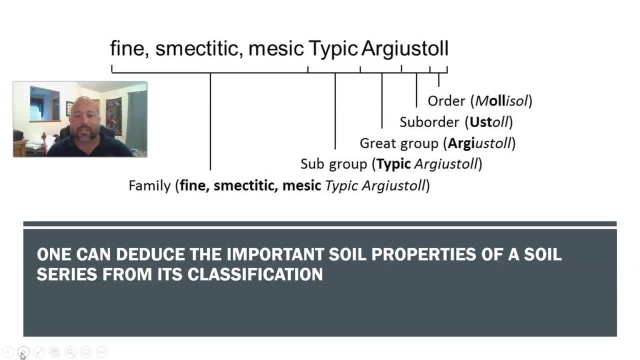 or coarse, so these are going to be more fine textured soils, smectitic. so it's going to have one of, it's going to have that two to one um kind of clay clay, uh content to it and then the um, the um kind of clay clay, then it'll be a very good material to have be within a um uh specific range. 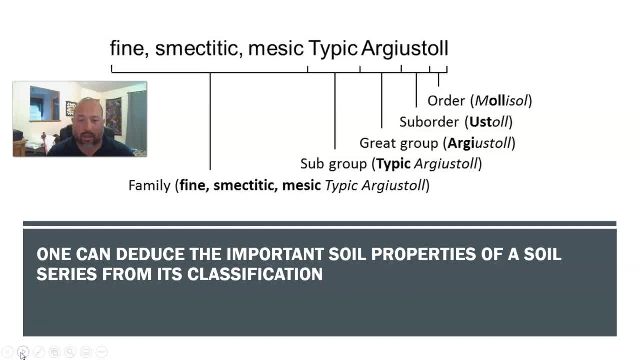 that would be related to that idea of smectitic and then the idea of um of mesic, in terms of um of the temperature range which i would just kind of describe as kind of mild uh temperatures. so fine, smectitic music, typical rgu stall. it sounds complicated but we actually know a whole bunch of information, if we understand, uh, these names and what they mean and what they can tell us. so, um, we know a whole bunch of information and then we know that we can find that there are things that we can. then if you don't find that, then it's still not a problem, but it doesn't make much sense because we can find that stuff. if we don't find that stuff, then it doesn't make much sense in terms of people that like to the information of the um of them and um, we have a bunch of information that we can find, the number of things that we can. 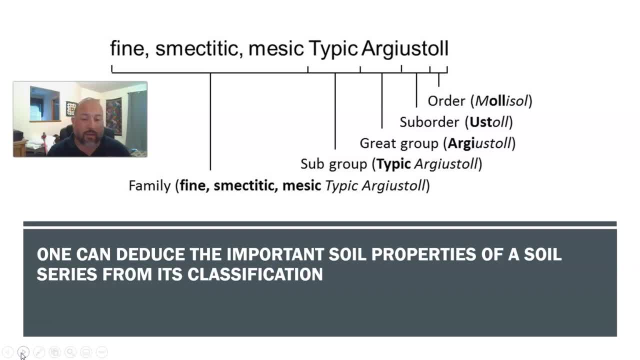 they can tell us and your book does a great job of having a bunch of different tables that really can help you with those different, those different prefixes and the different little names and adjectives and and what they actually mean. and if that doesn't work, just googling some.